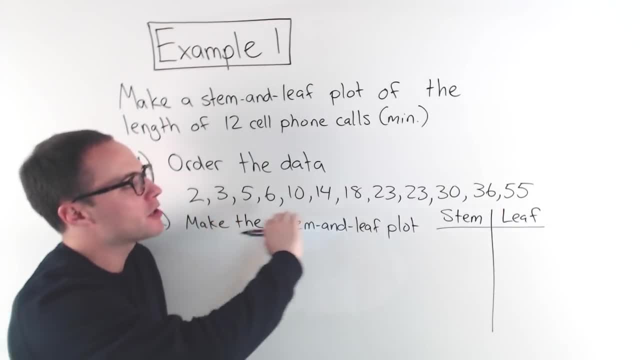 With that kind of range, I'm going to go by tens for my leaf. So first: well, 2, 3,, 5, 6, what do they have in the tens place? Well, it's not there, but you can put a zero there, right? 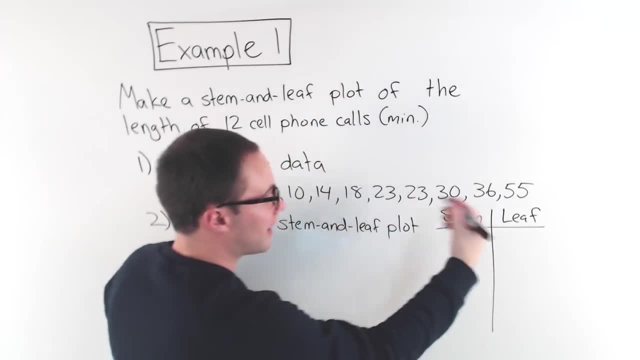 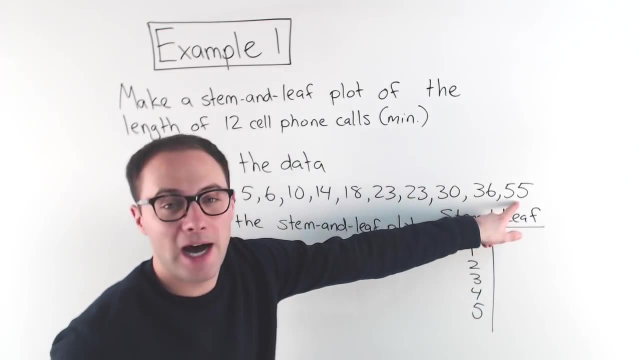 So that's a zero in the tens place. Then I go all the way up: 1,, 2,, 3,, 4, and 5, okay, 55 was my last value. That's the highest value. There's a 5 in the tens place, so I can stop there. 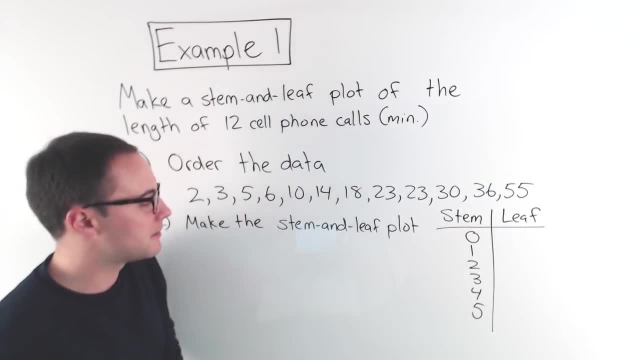 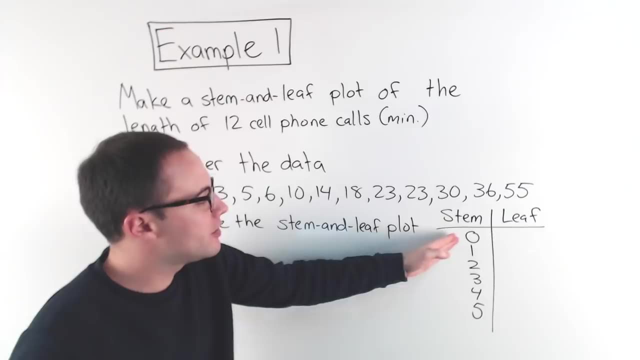 There's nothing. There were no phone calls that were 60 minutes and something Notice. I didn't skip any numbers. When you're making your stem and leaf plot, whatever you decide for your stems, you cannot skip any values, okay. 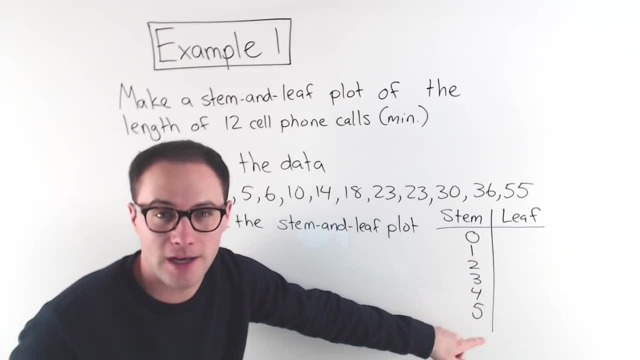 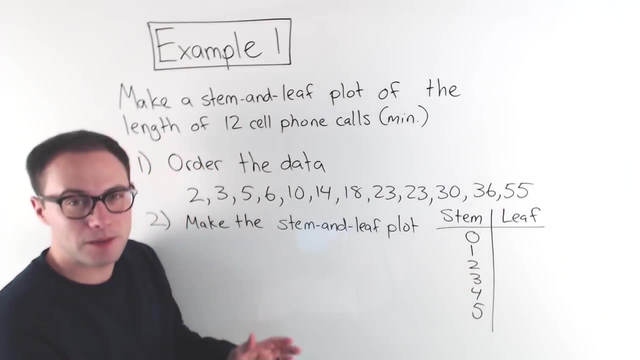 So I can't go 1,, 2,, 3, and then 4,, 5,, 6.. Even it doesn't matter if there's any values on that stem. It doesn't matter, You can't skip anything. 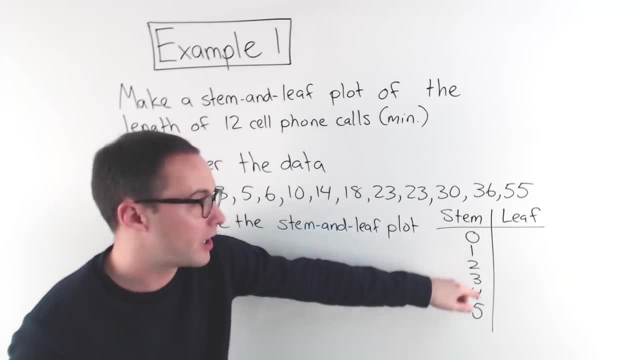 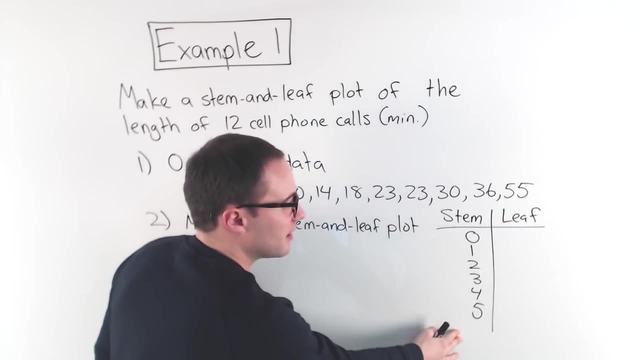 You got to go directly in order Until you're finished wherever you need to stop at the end. okay, So that's my stem. Now. this represents the tens place here. The leaf is representing my ones place. So look at your values. 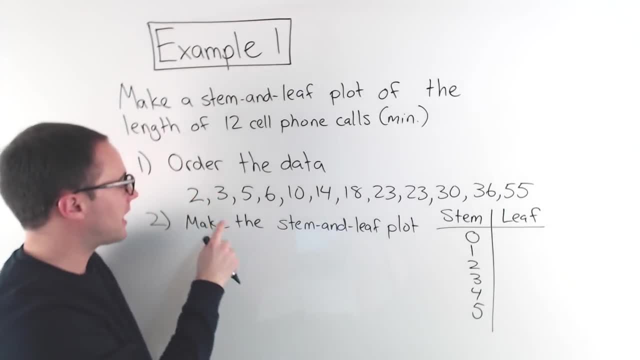 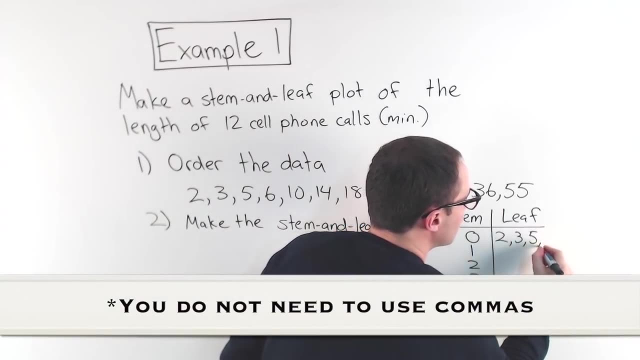 Well, for the values that have a zero in the tens place, I have a 2,, 3,, 5, and 6.. So we put those in order here: 2,, 3,, 5,, 6, okay. 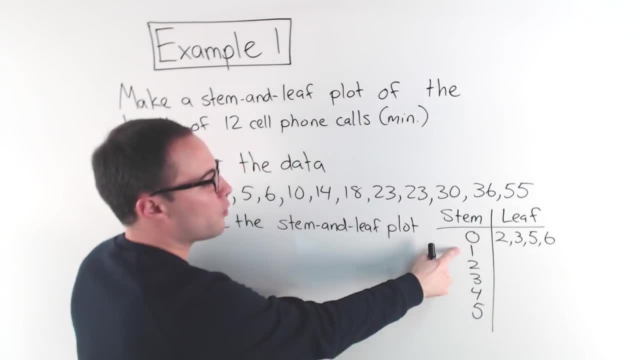 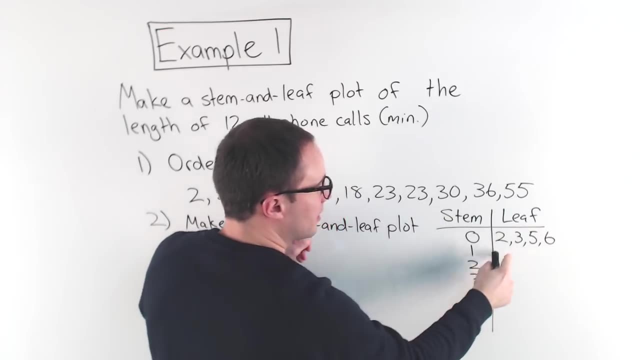 Just like that. Next, Well, what values? What values have a 1 in the tens place? Well, I've got the 10,, 14, and the 18.. So now I'm writing the ones value here for the leaf. 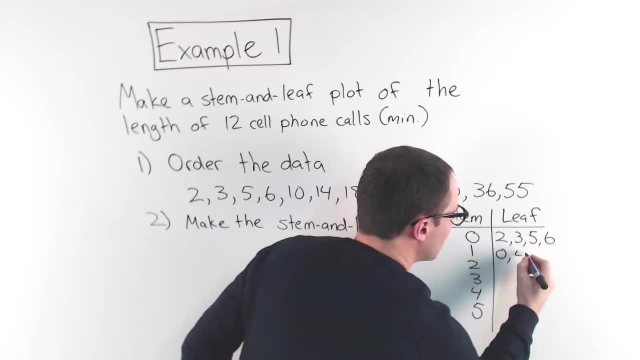 So I've got 0,, 4, and 8.. 0,, 4, 8. And we keep doing that. Well, I've got two 23s, So that would be 3, 3.. 30 is there's a 30.. 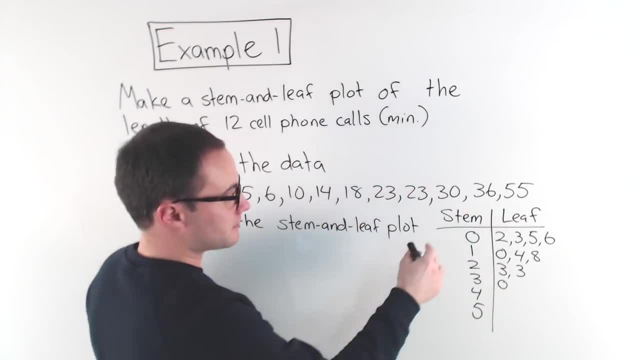 So I'm going to put a zero there. That represents 30. I also have a 36. So I put a 6.. Notice, there is no numbers in the 40s. okay, So do I put a zero there or leave it blank. 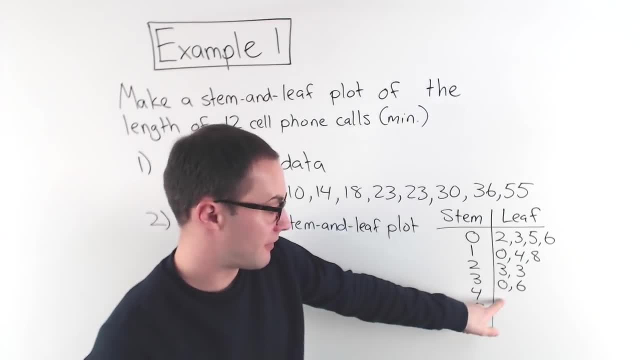 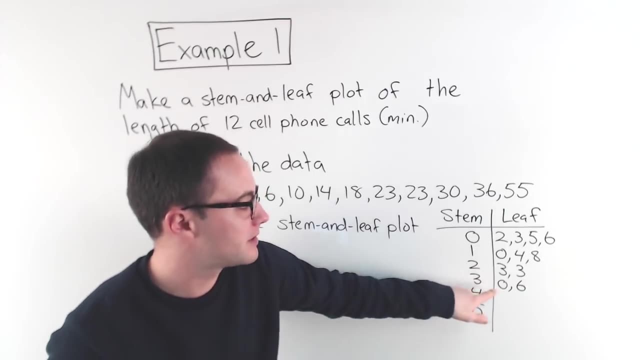 Well, if you said leave it blank, you're right. If I put a zero there, that would mean a phone call of 40 minutes, just like this zero here represented 30 minute phone call, But I don't have any phone calls in the 40s, so I leave it blank. 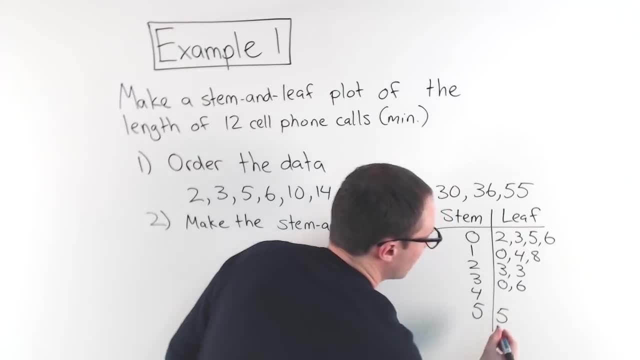 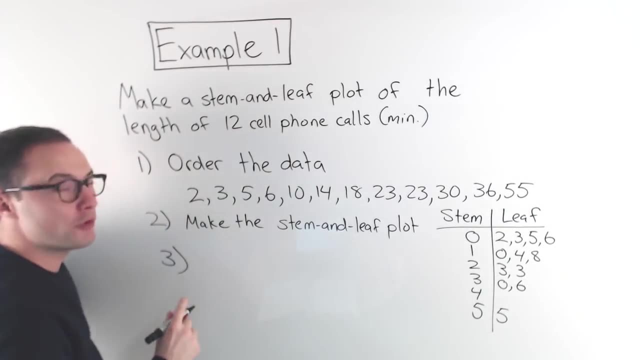 Go to the last one. I'm going to put a 5, so I'm going to put a 5 there. So this is my stem and leaf plot. We're almost done. Now step 3, really, really important not to forget this- is to make a key okay. 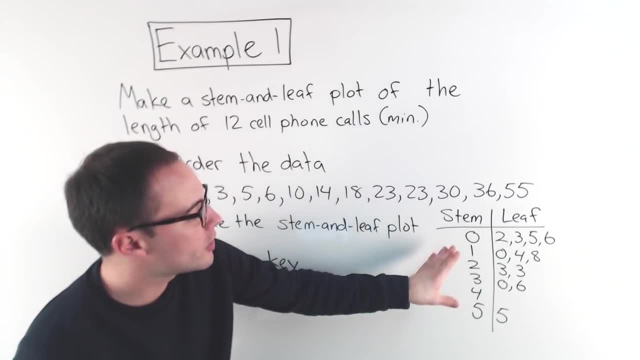 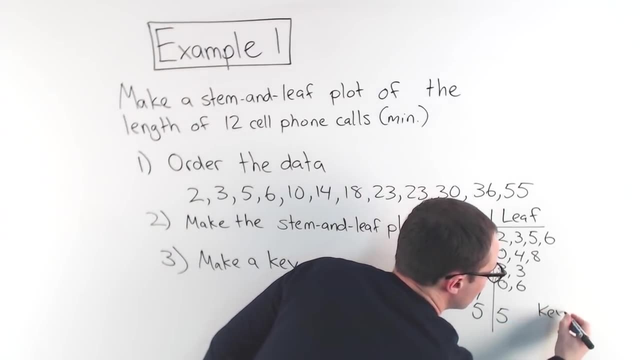 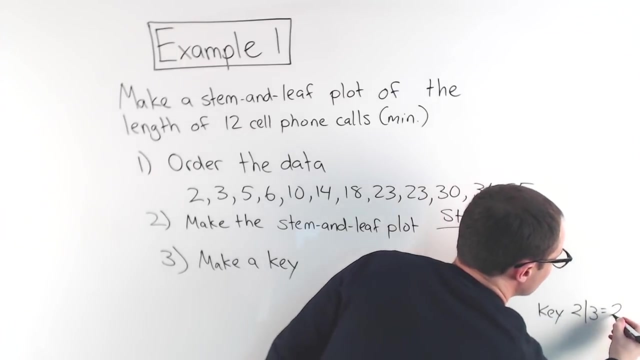 And the key is really, really important. Basically, all you do is you pick any example here for any value. I'm going to put the key over here. Hopefully you can see that okay. Yeah, So the key. let's say I'm going to do this: 2, 3, like that. so a stem of 2 and a leaf of 3, that means 23,. okay, 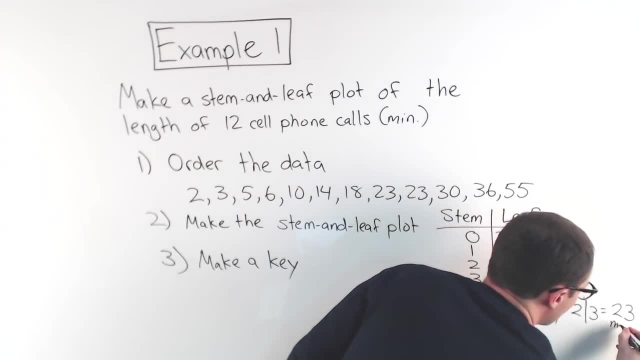 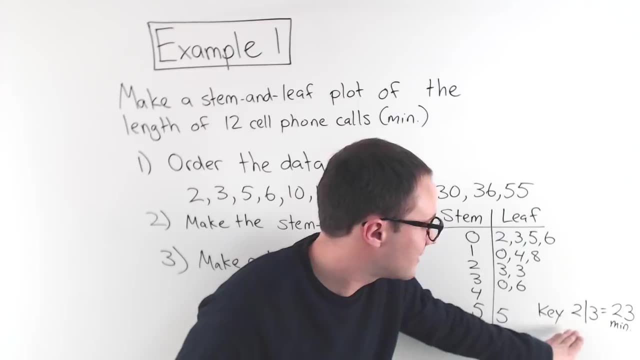 I guess I should put minutes too. I don't really have room, but 23 minutes okay. So that's my key. You can box it if you want or you don't need to, But the whole point is give an example from your data, okay. 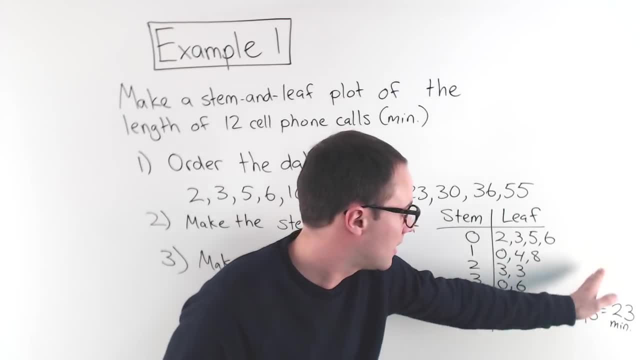 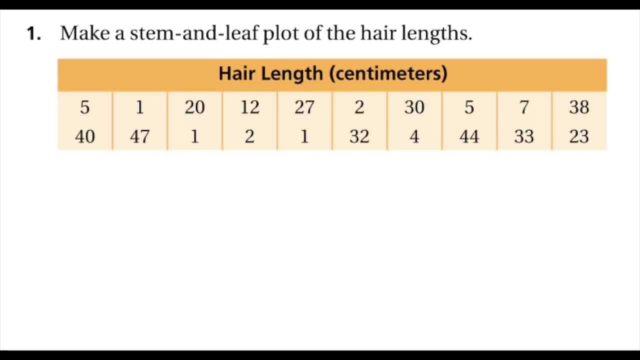 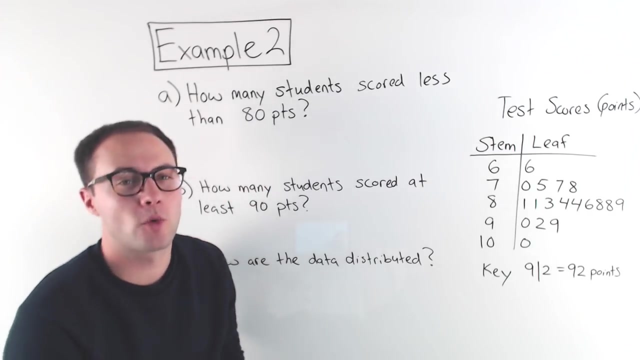 So that we know exactly what this Stem represents, and the leaf as well. okay, Good, Here's one to try on your own. Okay, example 2.. We've got three different questions. Notice we already have the stem and leaf plot over here. 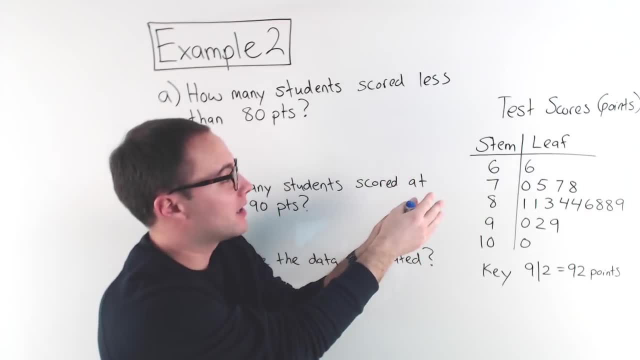 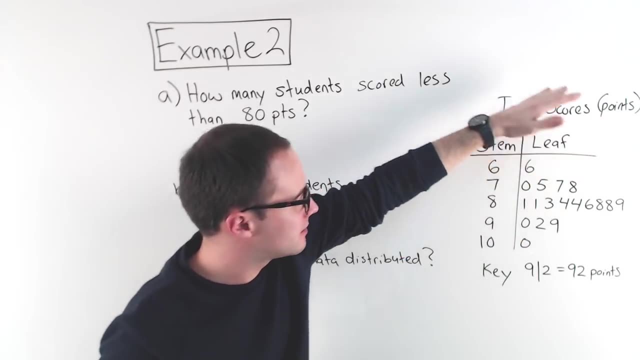 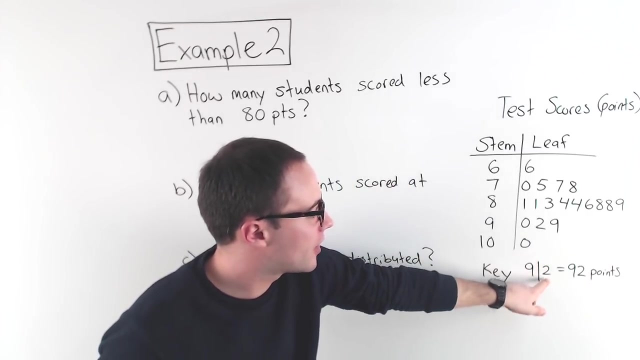 So instead of making it now, we're interpreting a stem and leaf plot. So let's just look over this real quick. The data is about test scores and points. How many points they got on a test score? Notice our key here: 9 for our stem and 2 for our leaf means that represents a 92, for 92 points on the test. 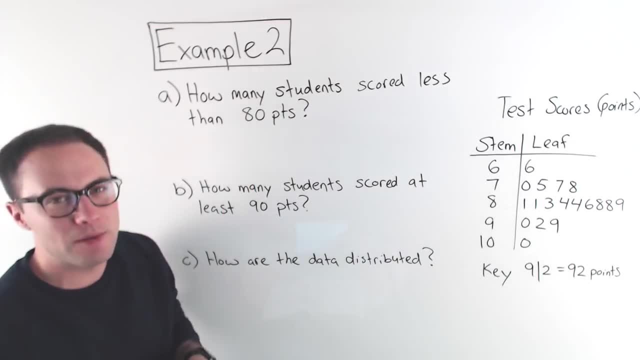 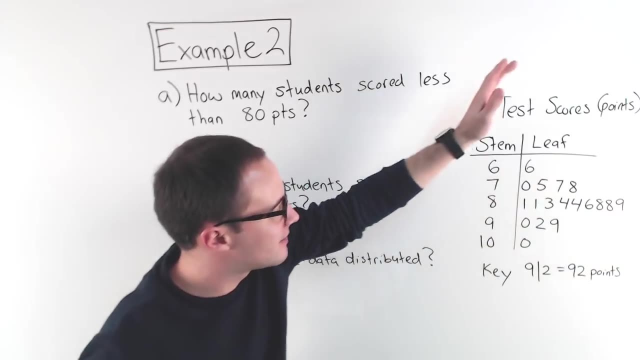 So let's look here. First one: how many students scored less than 80 points? Well, all of these here are in the 80-point range. Less than that. well, that would be a 78,, 77,, 75,, 70,, 66.. 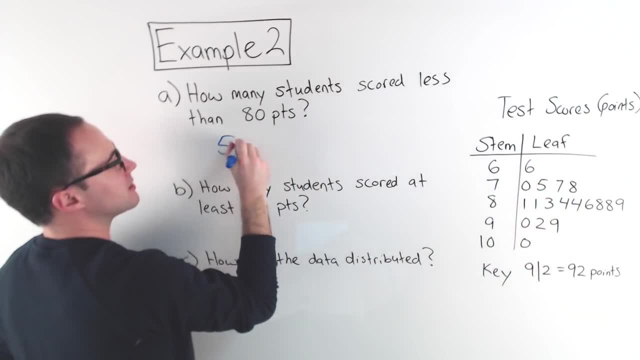 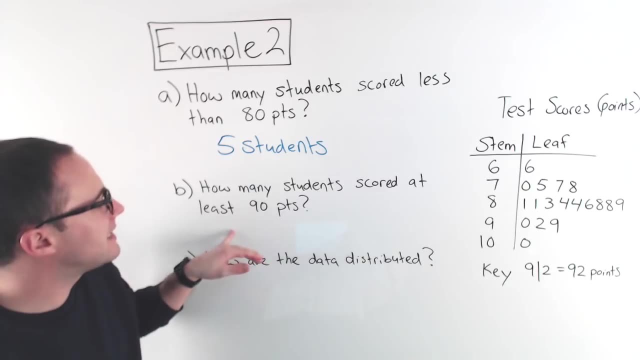 So we have 1,, 2,, 3,, 4,, 5.. 5 students scored less than 80 points. Next one B: How many students scored at least 90 points? At least, that means 90 points or greater. 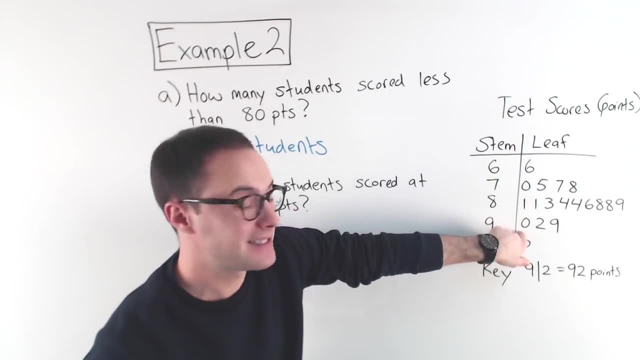 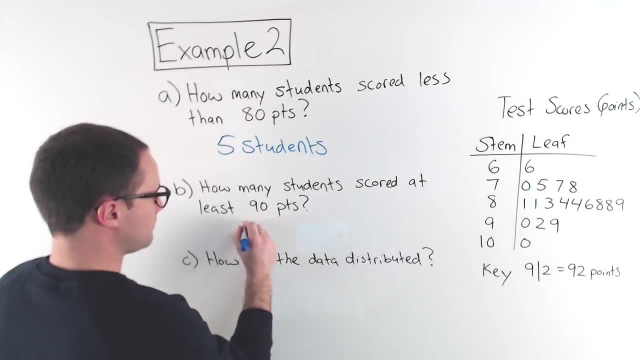 So let's see This: 0 here, that's 90 exactly. So there's 1,, 2,, 3, and 1 person got 100 points, So that's 4.. 4 students got at least 90 points. 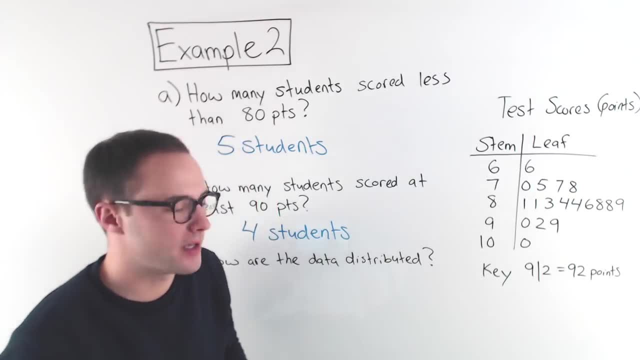 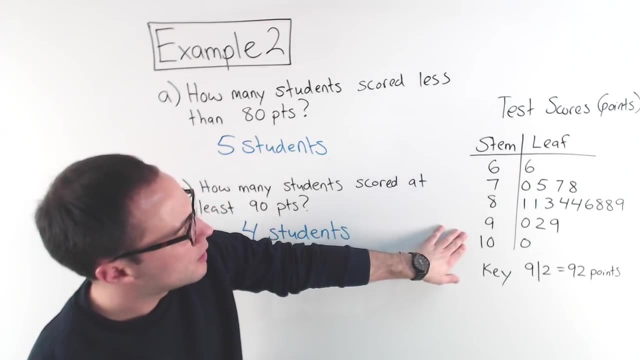 And the last one: how are the data distributed? So that just means what's kind of the shape or how is it spread out? So if you notice we have kind of a few, just kind of: 1 student was pretty low, 1 student was really high. 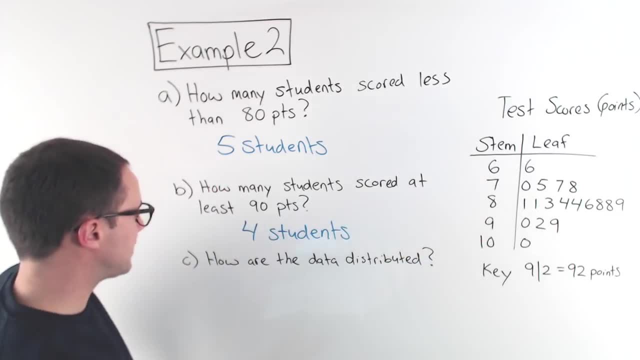 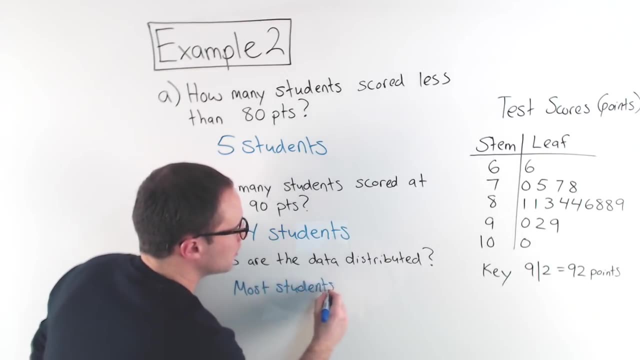 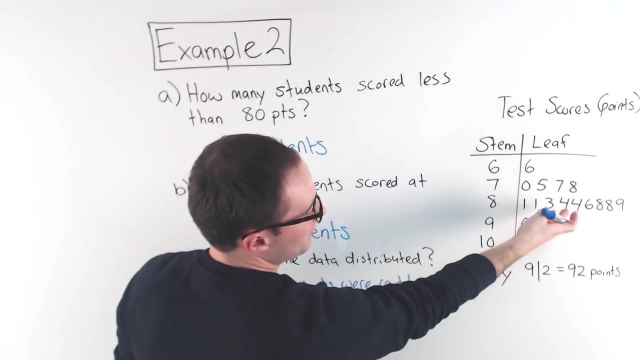 Everybody else is kind of in the middle, right? So let's say that. How are the data distributed? Most students were in the middle and we can say around. we can say around 80,, probably the exact middle, maybe around 80, 84 points. 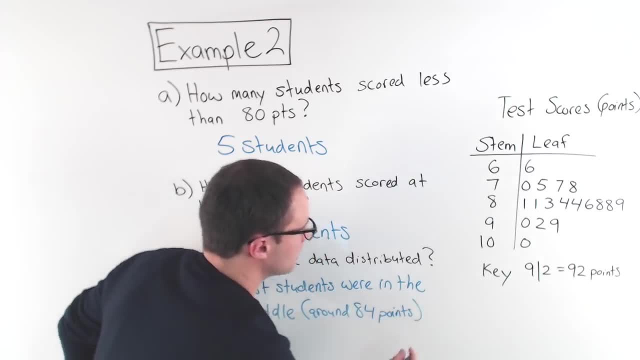 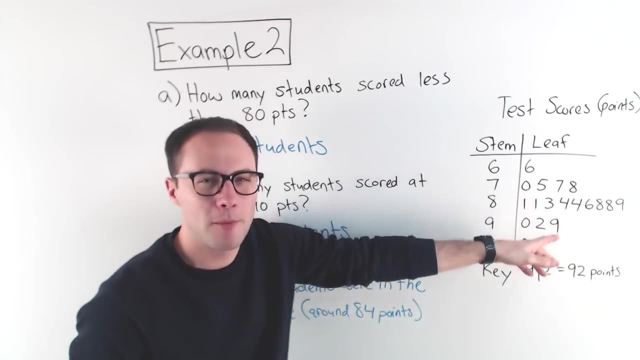 Whoops Around 84 points. Okay, Now one last thing. You'll notice with the stem and leaf plot. When I did the example before I put commas. You don't need to do that. I probably shouldn't have done that. 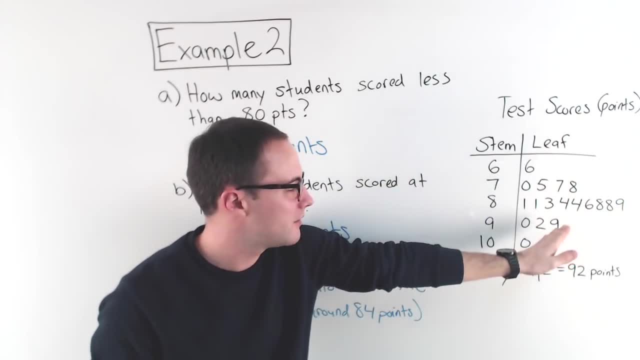 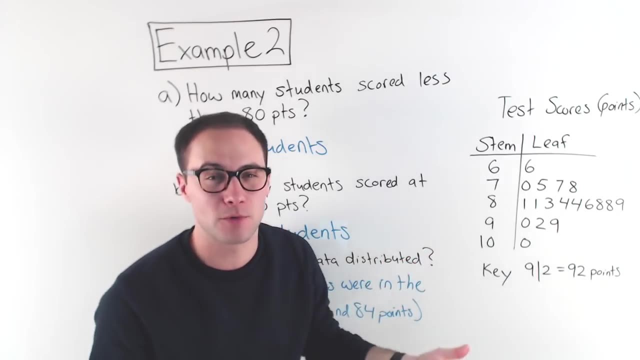 Notice here. all you need to really do is just list the numbers for the leaf, So don't worry about doing commas. And also, if you're wondering: well, can we use this for decimals? Like what if my data is decimals? 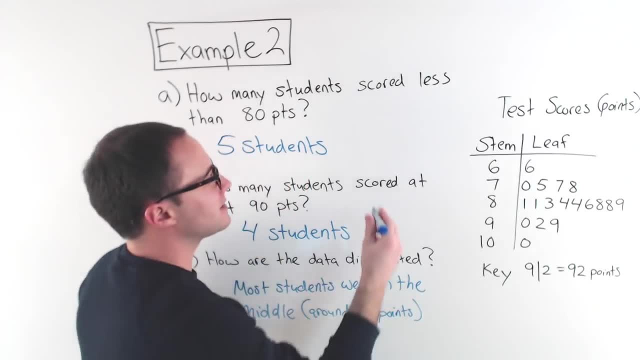 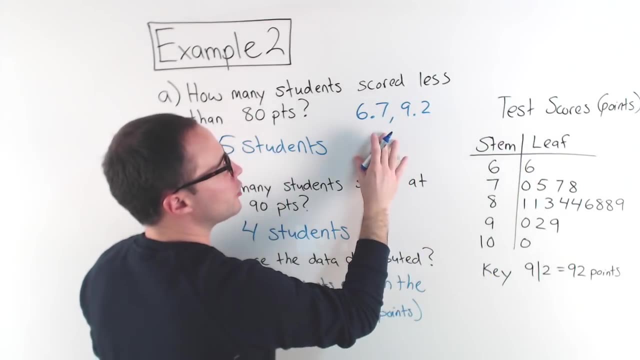 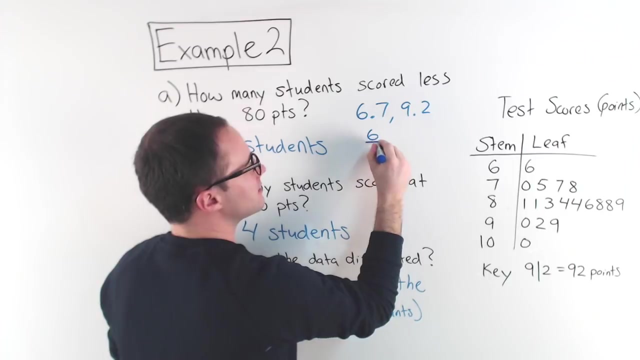 And yes, you can, And what it's going to look like. let's say you've got 6.7,, 9.2, and so on. Well, you can make it where this line represents the decimal point. So I could do something like 6,, 7,, 8,, 9 here. 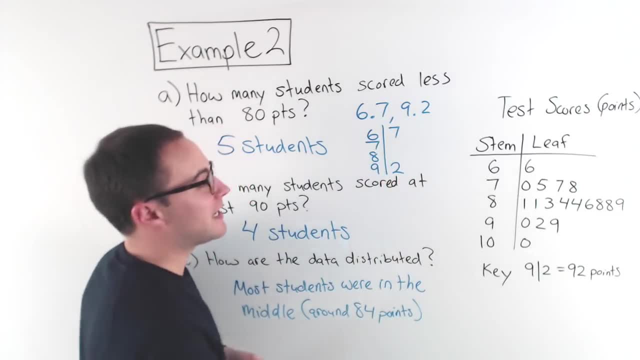 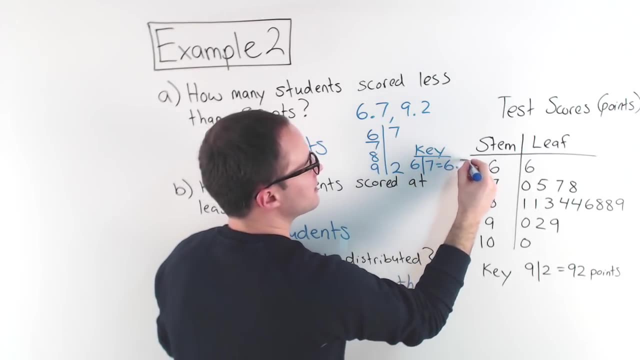 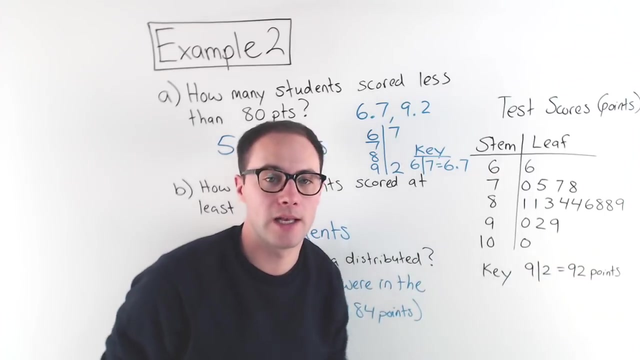 I put a 7 there, a 2 here, and then your key would be like: right, 6, that line, 7 equals 6.7.. Okay, that's why the key is so important, so that we know exactly what it's representing. 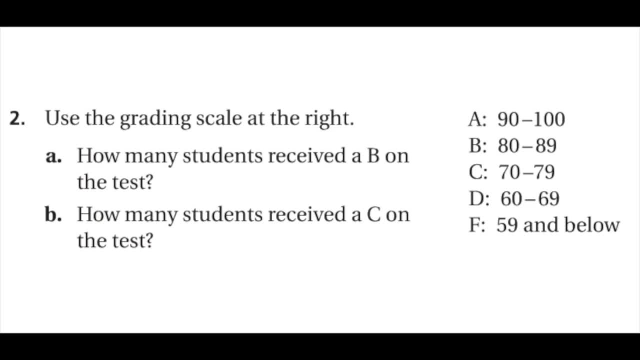 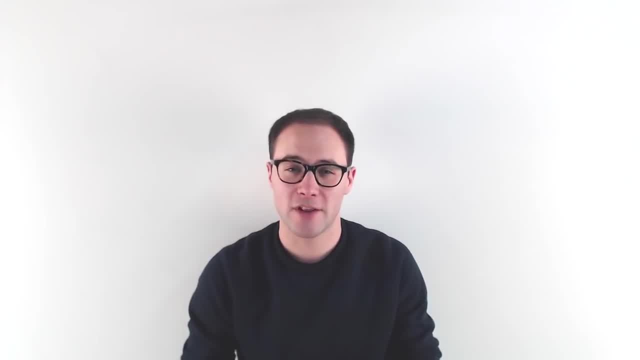 Okay, Here's one more to try on your own. Thank you so much for watching and if you like this video, please subscribe.